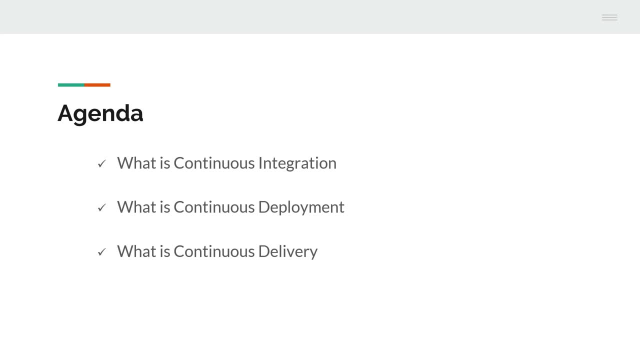 integration, continuous deployment and delivery in such a way that you will never forget this in your life. Okay, so let's not have any further delay and let's start with the first best practices. that is continuous integration. So what is continuous integration? So, if you 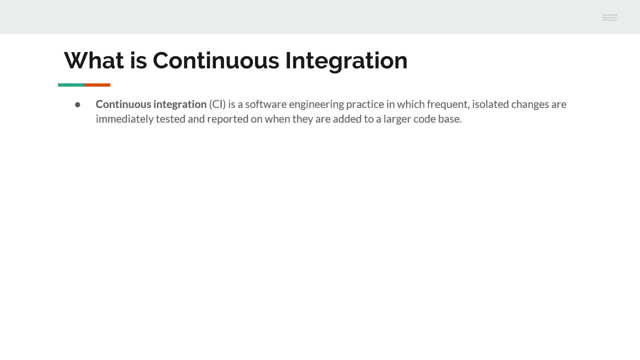 go with the internet definition. so continuous integration is a software engineering practice in which frequent isolated changes are immediately tested and report on when they added to a larger code base. So now let's cut this definition into parts, Part by part, and explain you every bit of it with a real time scenario. So this is the 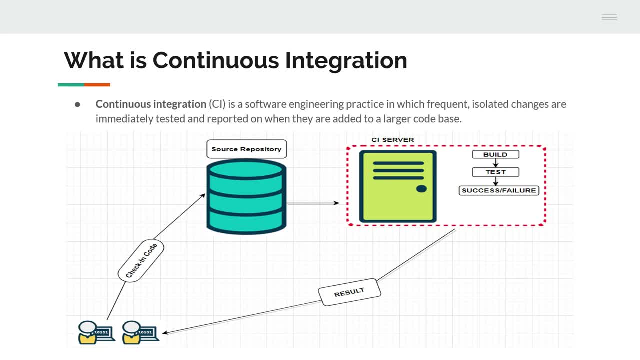 picture. This is a pictorial representation of continuous integration. So let's assume that you are a developer and you made a change. You made a code change in your source Java code, in your Java code, and you pushed that particular change to the central source code. 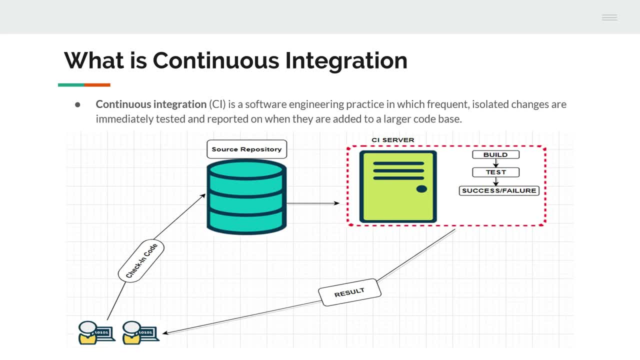 repository- Okay so that source code repository might be GitHub, GitLab or Perforce or anything. Okay, so once that code has been pushed, Code which is updated in the repository: Okay so the CI server will pull that change and start running it. So there are two parts of running. that is execution. There are two parts. 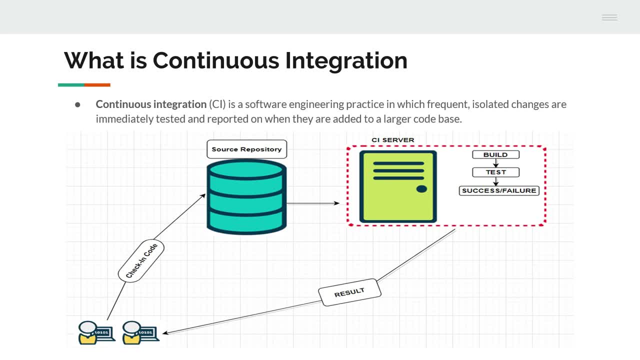 of execution will be performed. Okay, so one thing is the continuous building activity and the continuous testing activity. So you can see over here that we have built and then we have test. So let's start, I mean, let's understand what do we do in the building activity? 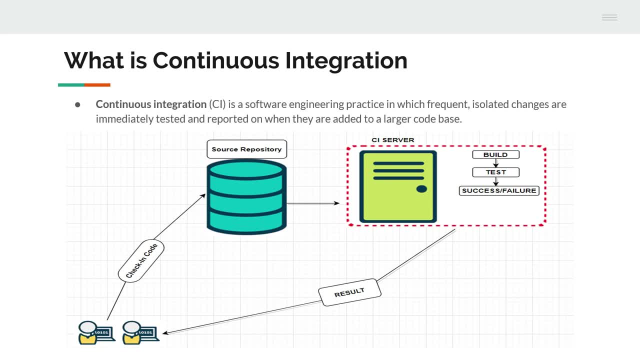 So, as part of the build activity, we will use any build tools To accomplish this step. okay, so, for example, like Maven, Gradle and all these are like build tools. okay, So once the build activity is done, the code will further used for the. 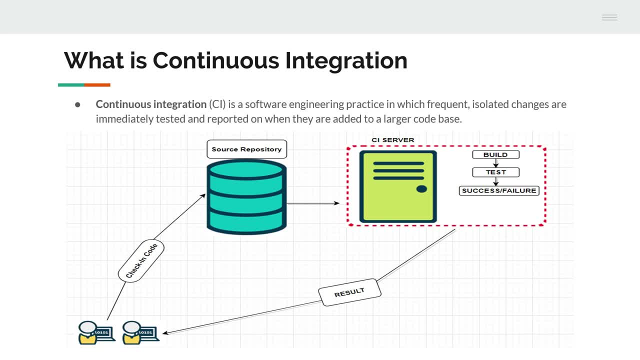 unit test as well as integration test, which is like written to test every line of the code. okay, So whether all the functionality in the Java class is working as per the expectations or not, so all these things will be tested over there. So in the case of Java, you might. 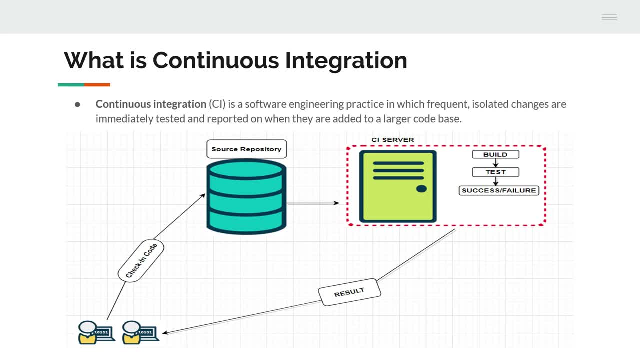 be running the Jaco co, that is, your Java code coverage. This is used to check the percentage of code being covered as part of the unit testing. Okay so, and then you might also have a predefined framework which will tell you that, which will. 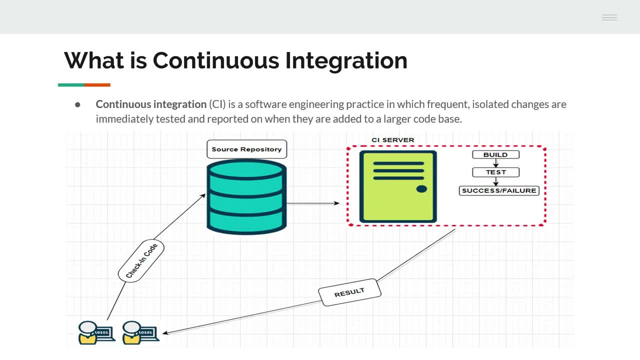 tell you the success rate of your code unit testing. So if your code unit testing success rate is more than 90%, then it will set. then the CI server will send an email notification to the developer with the required build artifacts which will be further use for deployment activities. 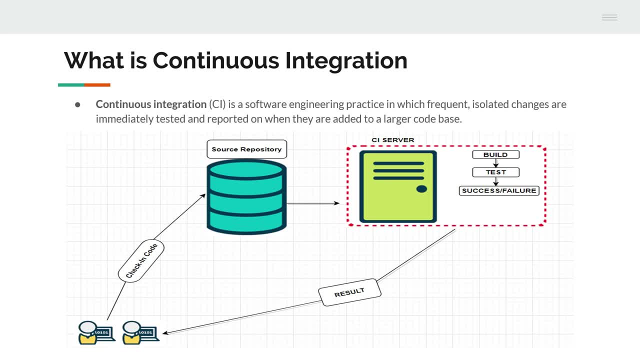 Okay. So now let's just understand from the developer perspective if they have to do all these activities manually. it is going to be a very tedious task, right? So hence CI will help. this. continuous integration will help you building and testing your code every time. 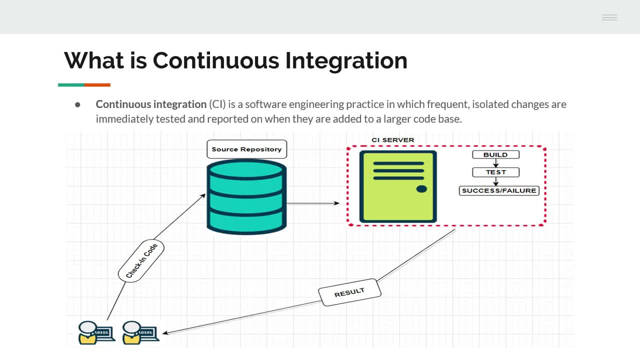 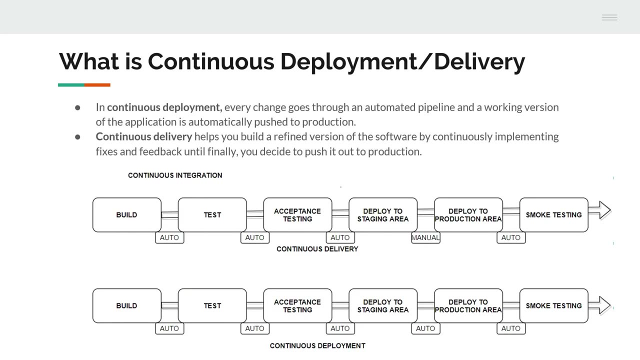 the developer checks in the code change in the source code repository. this is a best practices which will be automated every time the developer makes a change. Okay, so this is all about continuous integration. Okay, So the next thing is continuous deployment and continuous delivery. So, all these days, 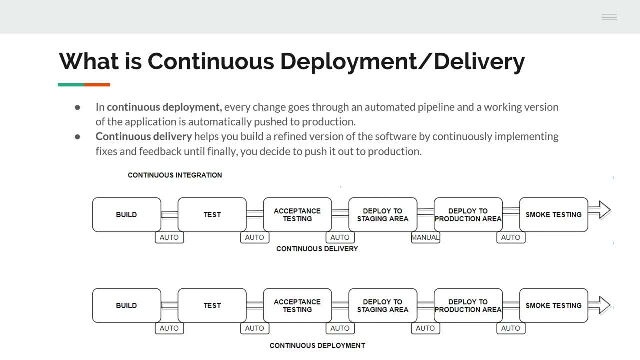 people are always confused between all both- both this definition- that many people use continuous deployment and they call it as continuous delivery. And many teams used continuous delivery and they still call it as continuous deployment. So these two are two different entity. okay, these two processes are completely different, So let's understand step by step. 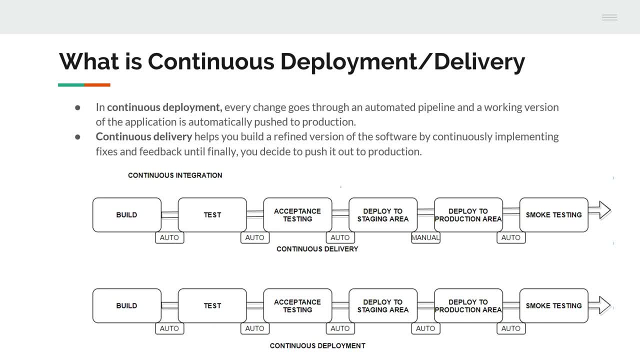 let's go with a definition: what is written in the internet? in continuous deployment, every changes goes through an automated pipeline and a working version of application is automatically pushed to the production. the below diagram is for the continuous deployment and the above one is for the continuous delivery. so let's start with the 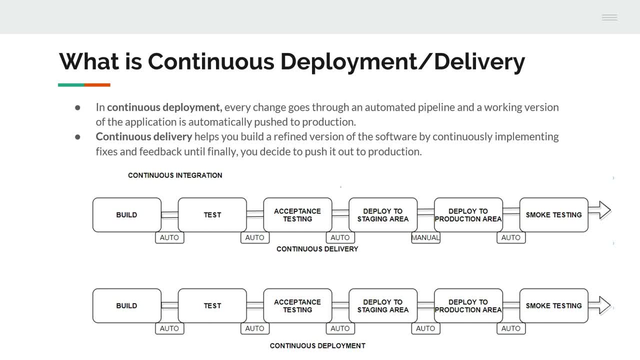 continuous deployment, deployment first. so again, this is also a software engineering practice. so the first two steps is build and test. these are the same step which continuous integration as part of the continuous integration, where, like the movement developer will make a change, the code will go for the build activity and then it will the unit and integration test will be. 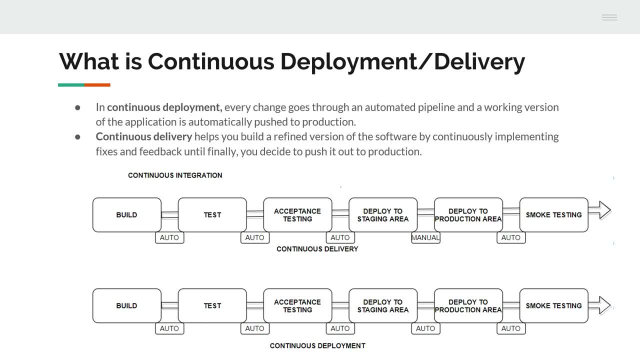 performed. so once this is done, the code package. so you will get a code package right that once the build activity is done, your code will be packaged with all the libraries and binaries and it will be packaged and it will be sent for the acceptance testing. so in this step, your code, artifacts or package will be tested with respect to performance. 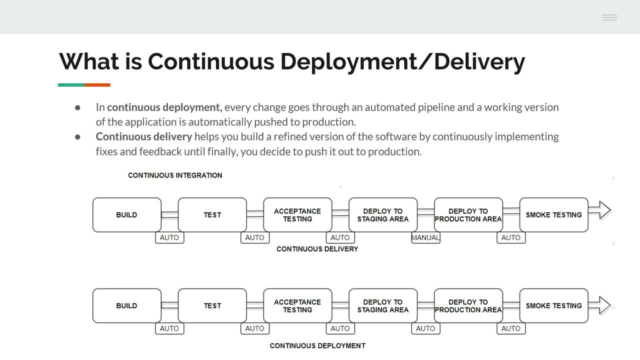 code, duplicates, code vulnerabilities, all the security aspects, etc. okay, so once we are fine with everything, i can say that my code is now ready to be shipped, but not directly to the production. okay, so you can understand that we cannot directly push the code to the production without testing it to, without testing in the local environments, though your 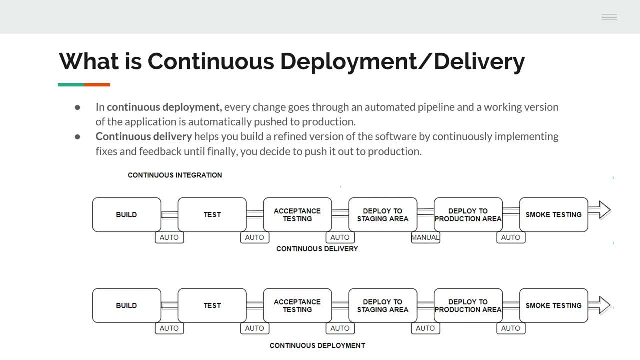 code doesn't have any issue, but you might be into integration related issues, okay, so hence, always we have to check in the staging areas first. so once it will be passed to the staging, it automatically goes and gets deployed in the production. once the production gets completed, we will just run some automated smoke test to test the 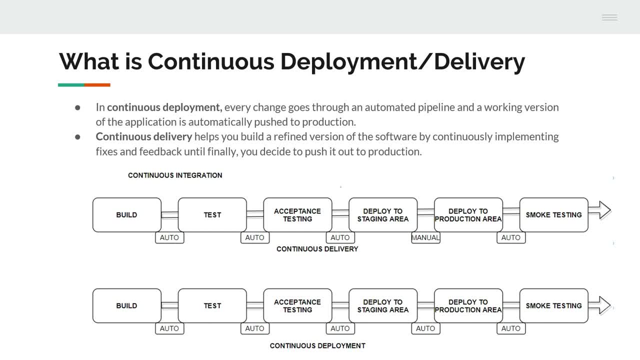 important functionalities, like in the case, for example, if we take the case of amazoncom, let's assume amazoncom is our project and so in if amazon is our project, we will change the login functionality. whether i'm able to add product in the cart or not, whether 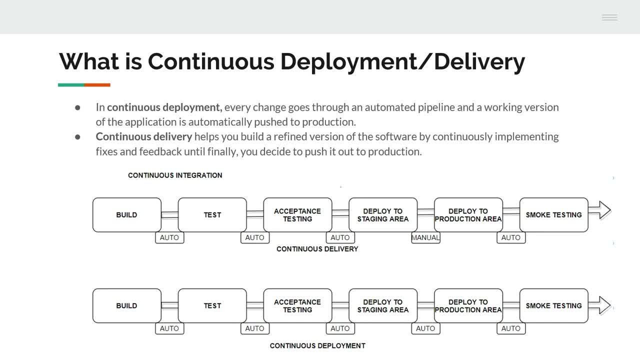 the checkout functionality is working properly or not. so all this active activity will be done automatically in the case of continuous deployment. so, for example, all this smoke testing via automation using selenium or qtp or any other tools. so so all these stages, like from build till the smoke testing in the in the case of continuous deployment, will be done automatically. there will 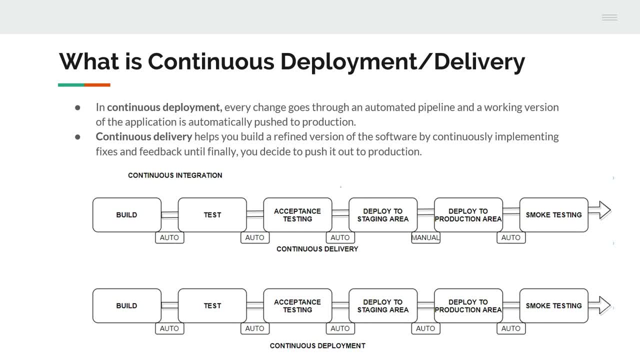 not be any manual intervention. okay, so now let's go to the continuous delivery. so continuous delivery is again a similar process where almost all the processes are automated, but there will be a manual approver before deploying, deploying anything, any feature change to the production. okay, so now i'll. 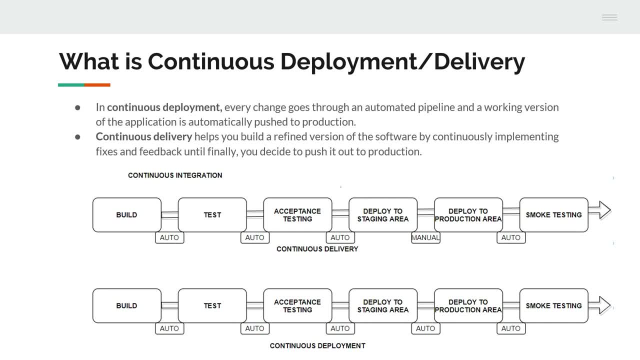 tell you why we do this. okay, so there are companies. there are companies where not all their services are running with zero downtime. so i mean all these companies take their own feasible time when their usage of the product is less, for instance, if most of the customers for that particular product is. 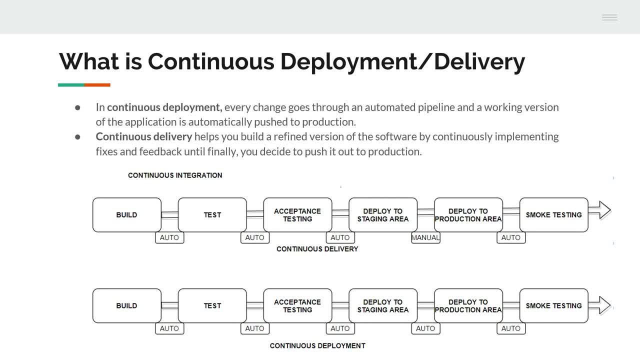 from usa. they will use the time to deploy and deploy the feature change into production when the entire the is slipping, okay. so again, i mean they will also update in their slack channel, the jira blog, as a notification to all the customers and client if they are using the products.